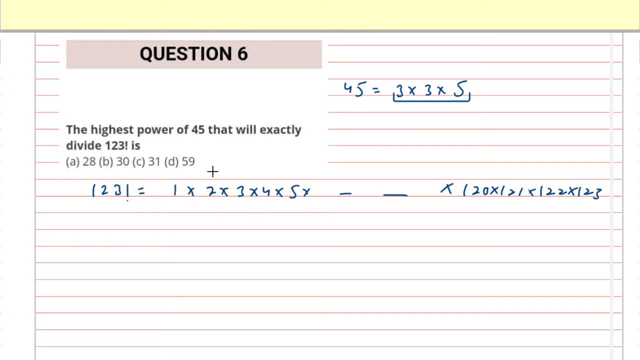 Then we will know the power of 45, that will exactly divide it. For that we have to count 3 x 3 x 4 x 5. First we will talk about the multiple of 3. If we see the multiple of 3, 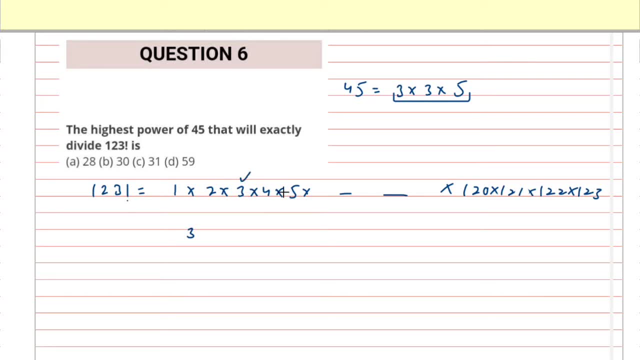 If we see the multiple of 3, So 3 will start from 3 and then 6 will come, Then 9 will come, So up to 123. If we divide 123 by 3, we get 41. This means there are 41 numbers which are multiple of 3. 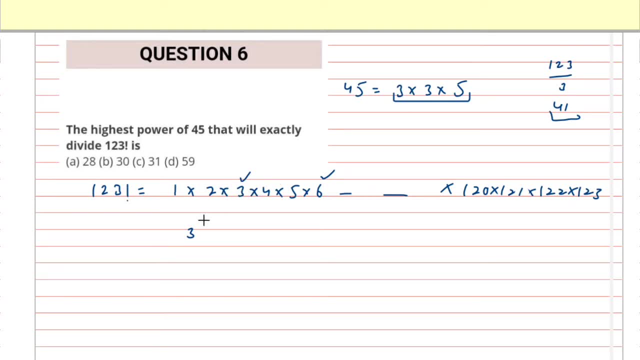 So we can divide all the numbers by 3 And we can say that 3 can be divided into all the numbers. So in total we have to get 3 x 41. So if we take 3 x 3 x, 4 x, 5 x, 5 x 6, we will get 41. 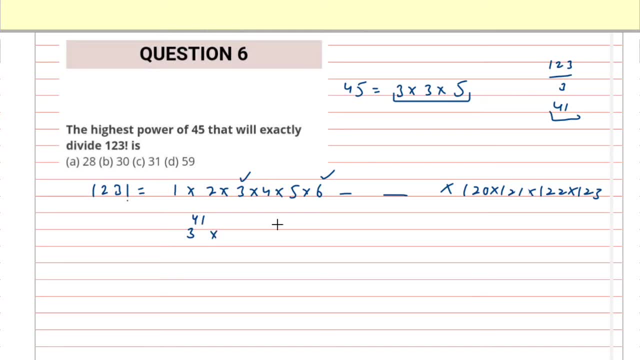 So we have 41 in 3 x 3 x 5 x 5. After this some numbers will be in the same way as the multiples of 9. So if we take 1 x 3 x 4 x, 5 x 6, we will get 1 x 3 x 4 x, 5 x 6. 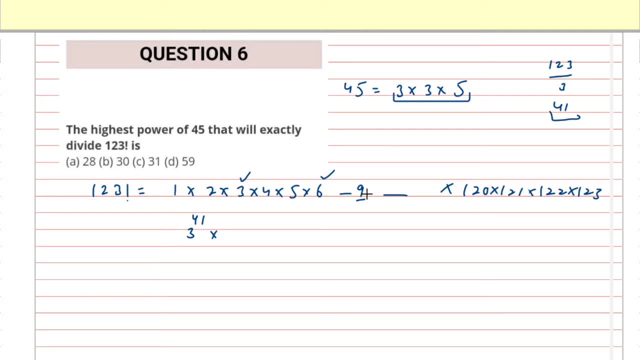 So we can say that 1 x 3 x, 5 x, 5 x 6, we will get 1 x 3 x, 5 x 7, So out of all the multiples of 9, 1 x 3 x, 4 x, 5 x 6 will come. 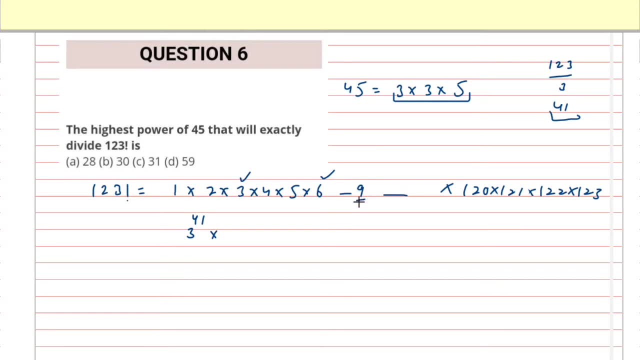 And the remaining 3 will also be counted. So how many are the total multiples of 9?? We have to divide 123 by 9, So 9 x 1 x 9 x 9 x 3 x 7 x 6. 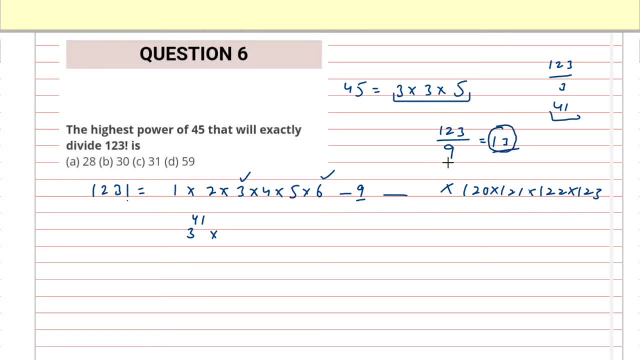 So we have 13 numbers, which are the multiples of 9. So instead of 1 x 3 x 4 x 5 x 6, we have 2 x 3 x 4 x 5 x 6. if we want this, we can divide this by 2, so 1 x 3 will be here. 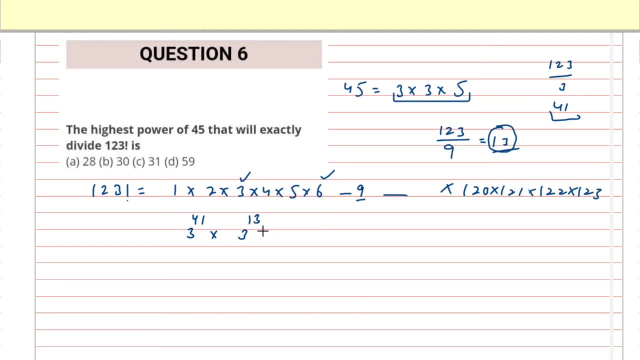 So 13 x 3 x 3 x 4 x 6, we can divide this by 2. After this we will have 9 plus 3 is 27. Now if we have 123 in the total, We can count 27 as 4. 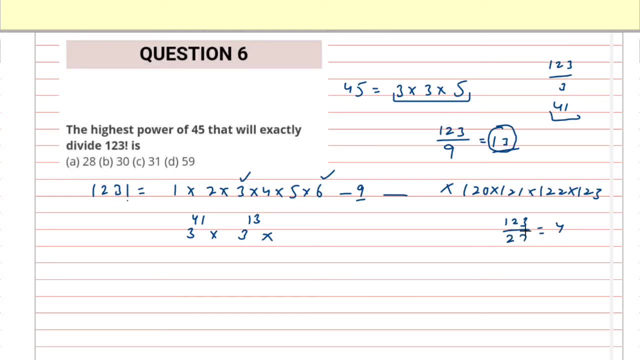 Because if we do not do 8, it becomes 108. After that we will have 123. Now we will have 123 in the total. So 4 numbers are divisible by 27.. So we can divide 3 by 3 and then divide 3 by 3.. 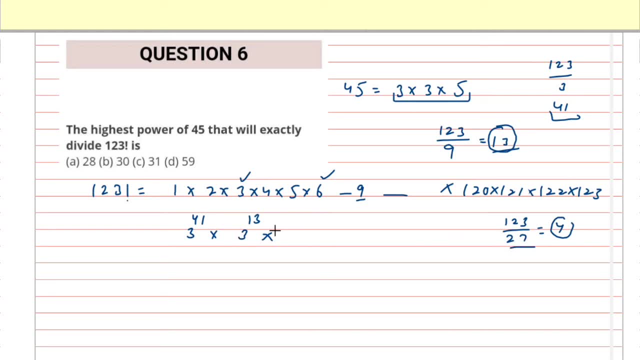 Because we can write 3x3x3 in 27.. So we can write 4x3x3.. So the total number of 3 is 58.. 3 raised to the power, 58. So the prime factorization of every number we can divide 58 by 3.. 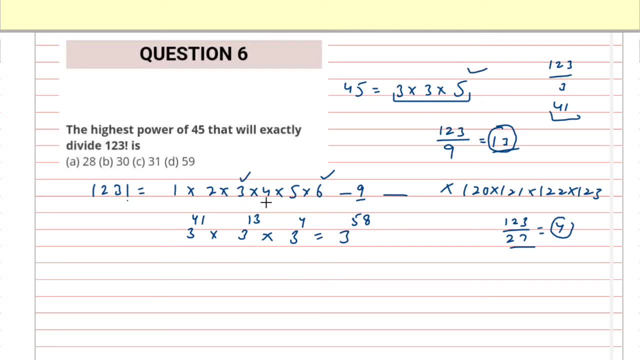 After this we will talk about 5.. So how many numbers can we write in 5?? First of all, we have to know the multiples of 5.. The multiples of 5 are 12. 24. 24. 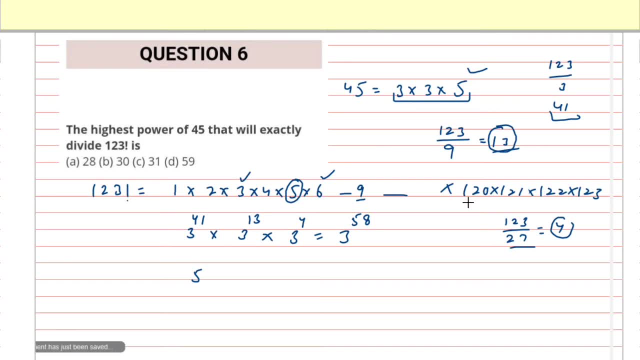 Because the last number is divisible by 5.. So we have to know 24 numbers, From which we can take 5 as a factor. After this, we have to know the multiples of 25.. As we have seen in the first part, 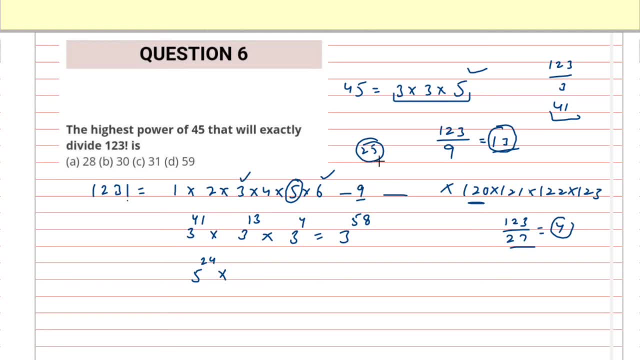 we have to know the multiples of 3,, 9,, 27.. So we have to know the multiples of 25.. So we have to know the multiples of 1,, 23,, 25.. So this is the last number. 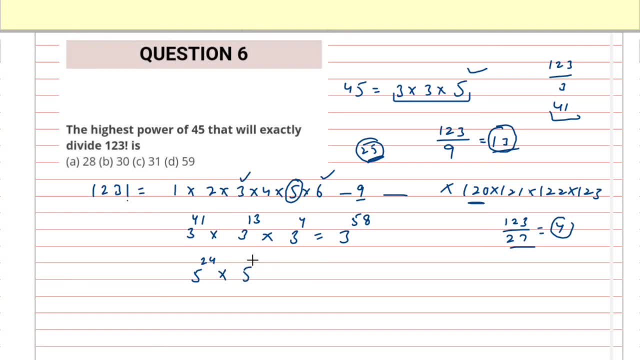 Then fourth is only 4.. The last number is 100. So we can take one by 4.. So after 25, we have to know the number 5 raised to the power 3.. Thus we have to know 1, 25.. 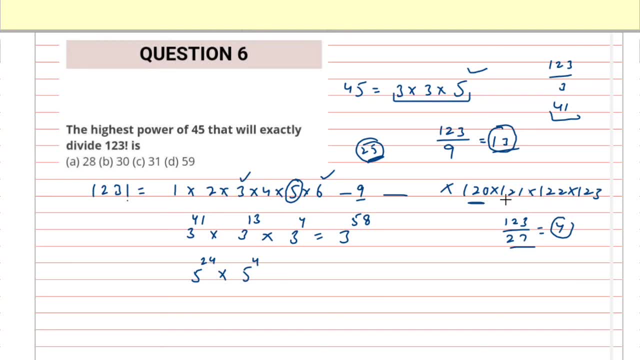 So the maximum number is 100.. The two 5 numbers that can be added We have to count them one by one. So what is the total number of 5 in this particular factor 5 raised to the power 28.. 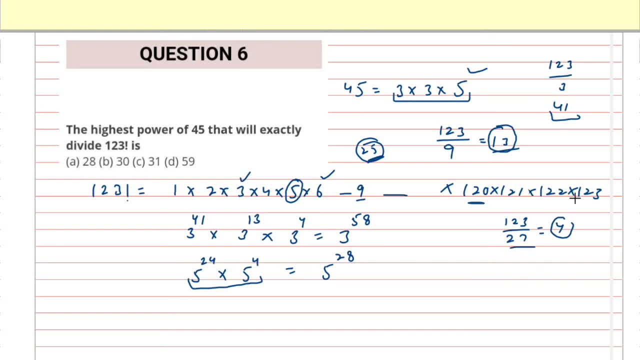 28 times 5 will be equal to if we did all this prime factorization. So now we need the numbers. We need 2, 3.. And we need 1, 5.. 2, 3, and 1, 5..